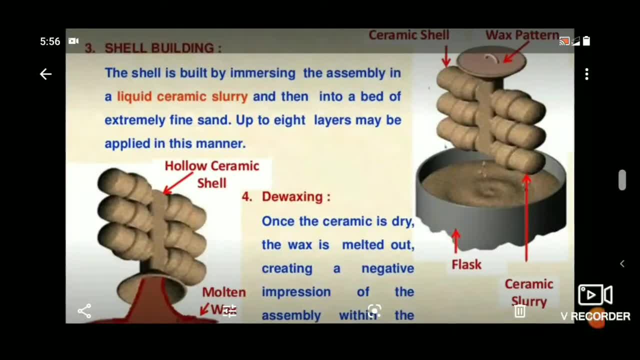 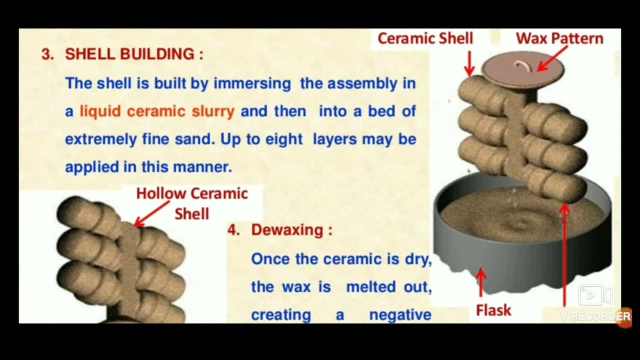 wax, then Shell building. to make the wax strong, we have to ensure that the wax, the outer surface of the wax, should be hard. for that we take a liquid ceramic slurry in a container and we dip the wax pattern assembly into it so that the wax surface gets coated with this liquid ceramic slurry and then de-waxing. 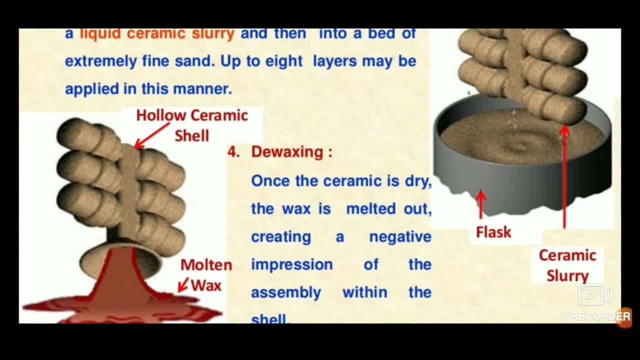 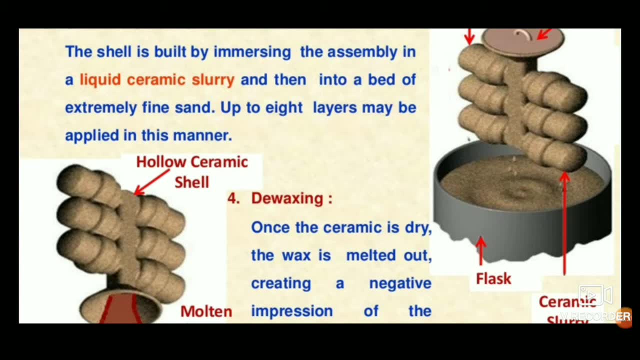 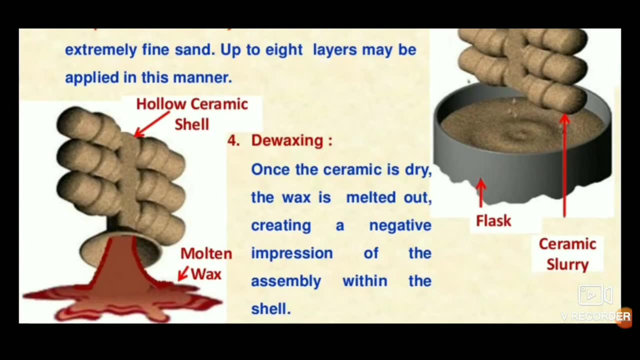 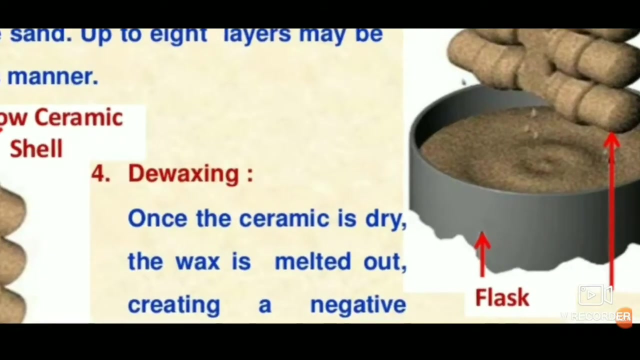 because de-waxing is an essential part. if molten metal is poured before de-waxing, the shape- accurate shape- cannot be achieved, so that de-waxing is made at that time. the wax is melted out using some heat so that the outer surface ceramic coating is only available in the assembly. then 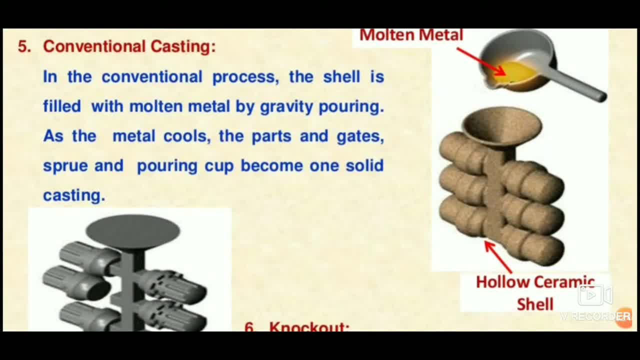 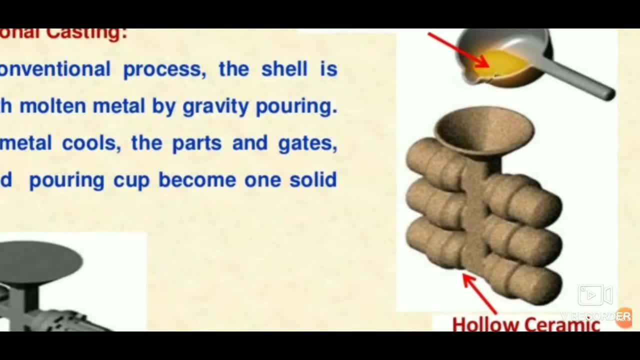 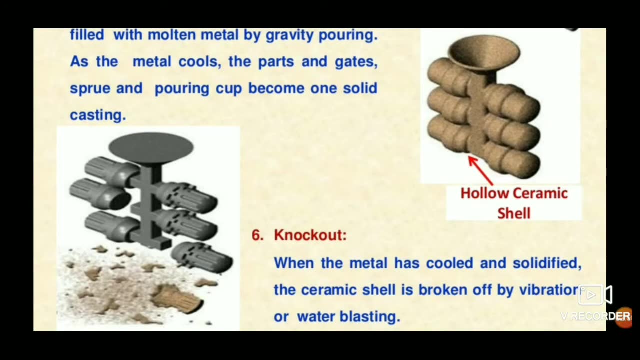 conventional casting, the molten metal is taken out and fill it over the sprue. and the molten metal goes inside the internal surface and gets filled up, then knockout. after cooling the ceramic shell surface, the outer covering is removed by vibrating or water blasting so that this outer ceramic shell is cleared out and finally the inside cold. 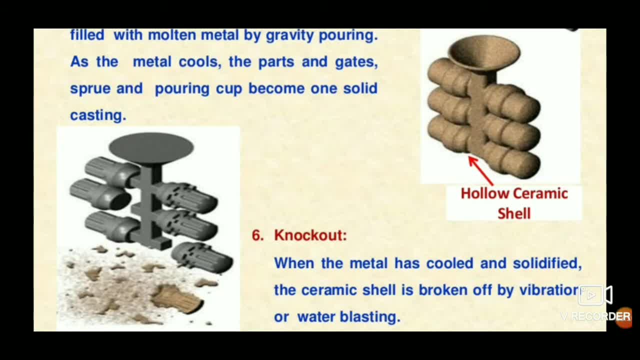 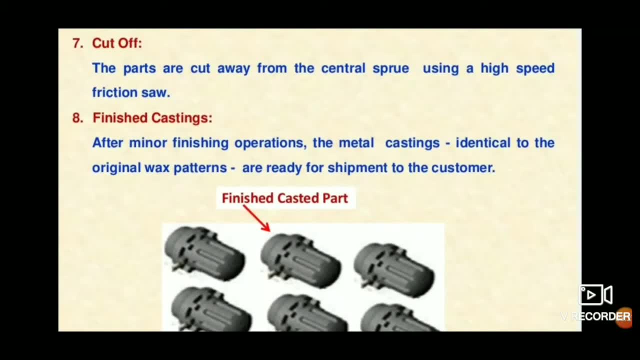 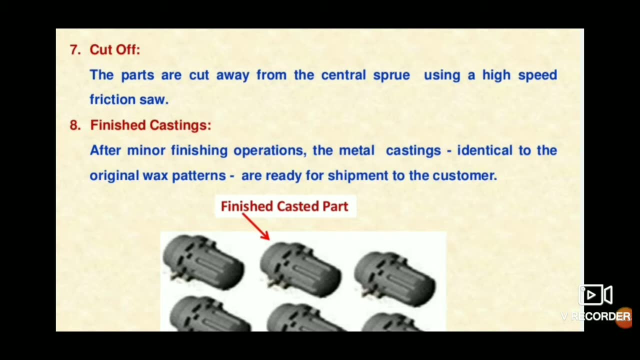 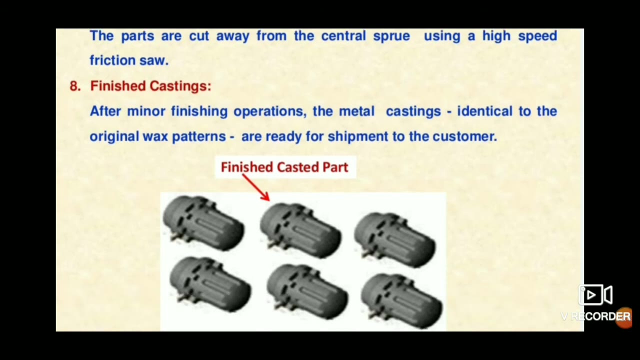 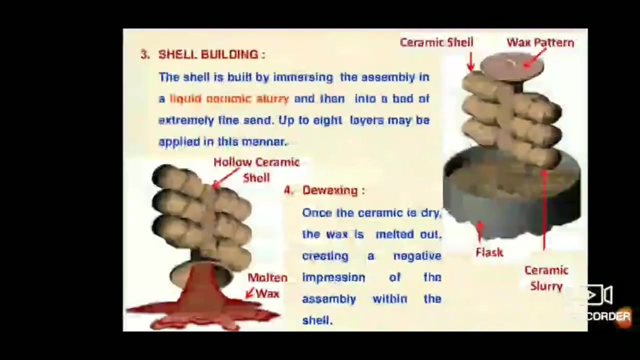 molten metal cold. the molten metal is cold and final product is having then cut off some gates- sprues are also- are always sticker together the assembled product so that we want to cut the sprue gating system etc. finally, the finished castings. that is the wax pattern that we have already made. this. 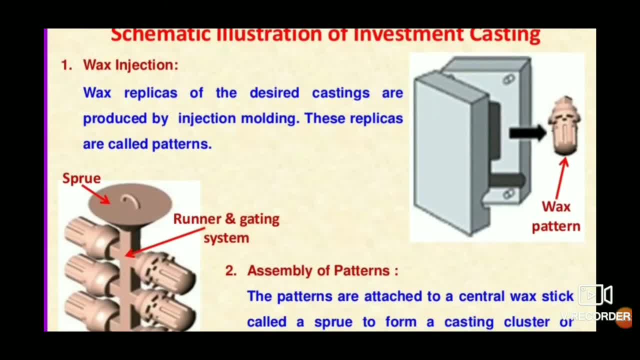 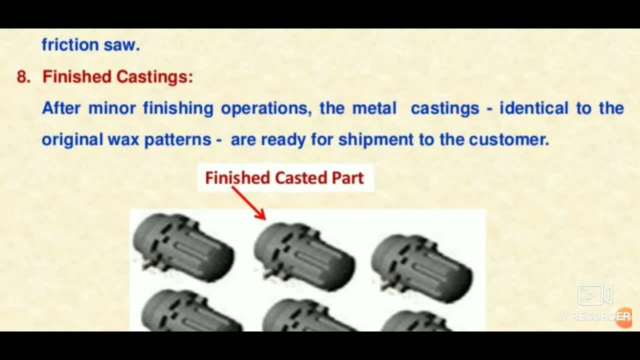 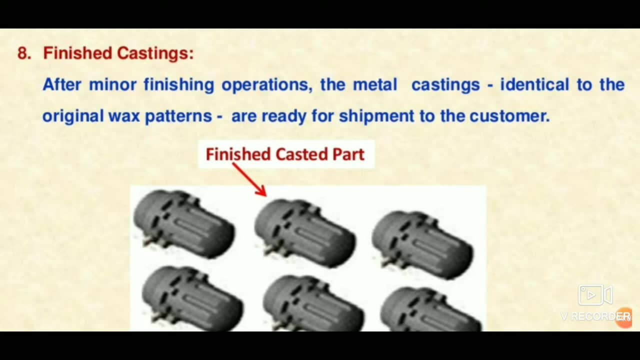 is the wax pattern. this is our product. so it is finally achieved in this process. after minor finishing operations like a cleaning, the mix of wax that stick on together on the molten metal, it can be removed and finally our finished to castor part is available. so